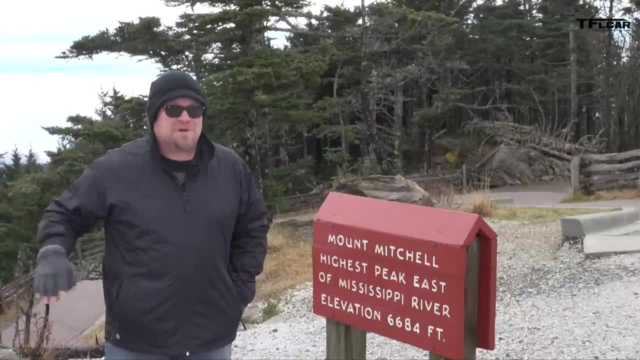 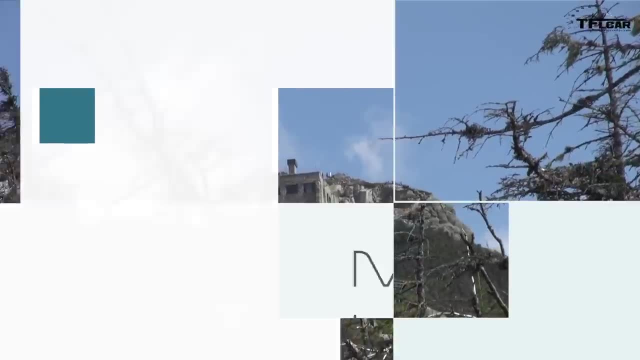 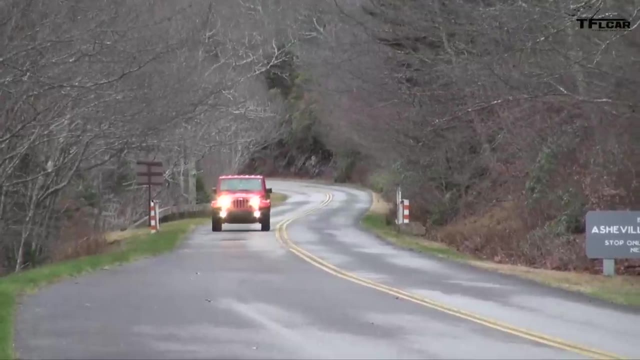 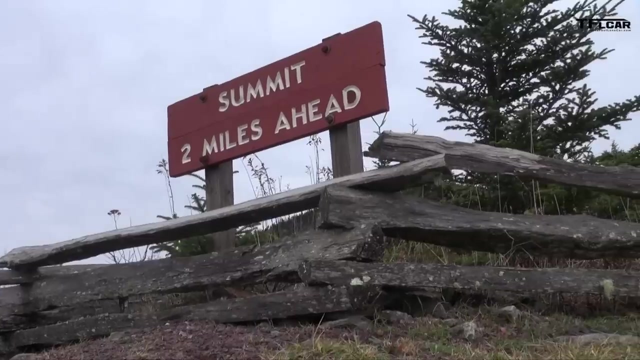 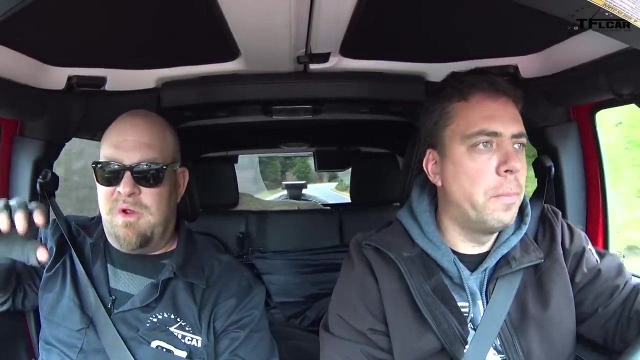 River and south of Canada, And coming up next we're going to show you this extraordinary park. Oh yeah, yay, cryptic. We've been talking, when the camera was up, like what would be the perfect car to come up this route, and here's where our head is. So I was thinking something along the lines. 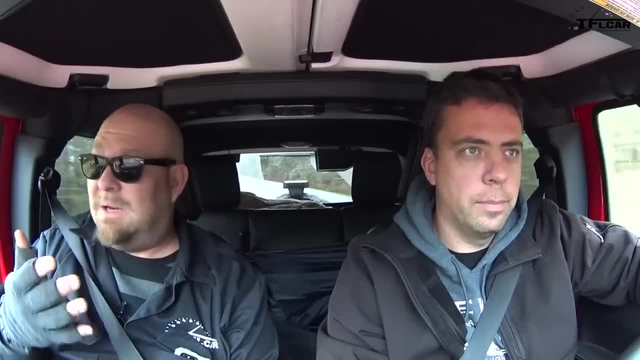 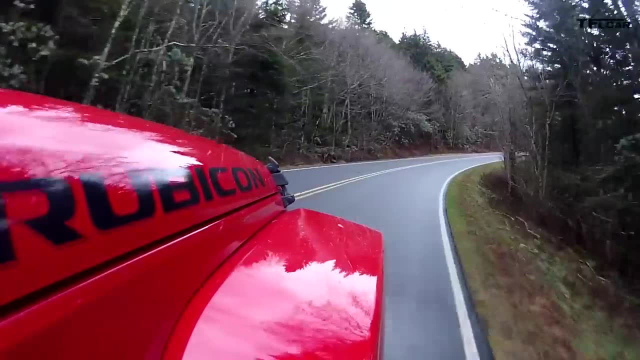 of the Fiat 500 Abarth. I think that would be just a load of fun here, Just hearing that engine crackle as you're just powering through the corners and, you know, going to maximum revs. The new Fiat 124 Roadster. 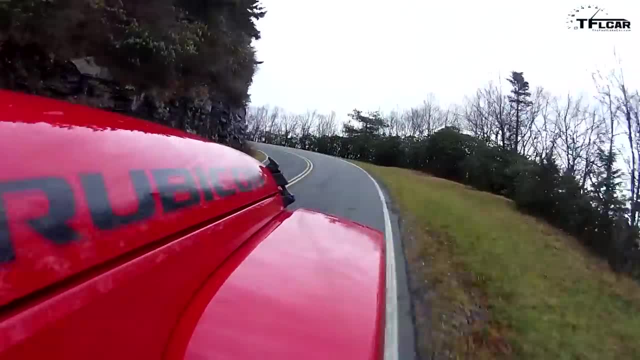 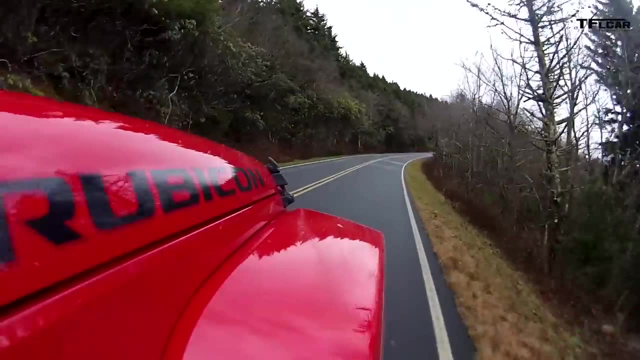 That ought to be interesting. Along the same line, Hell yeah, That ought to be fun. Which, of course, just like the Mazda Miata, although with the Fiat it has the Abarth engine, which we are absolutely in love with. 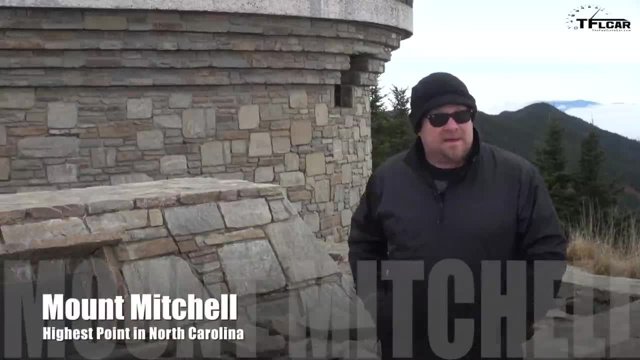 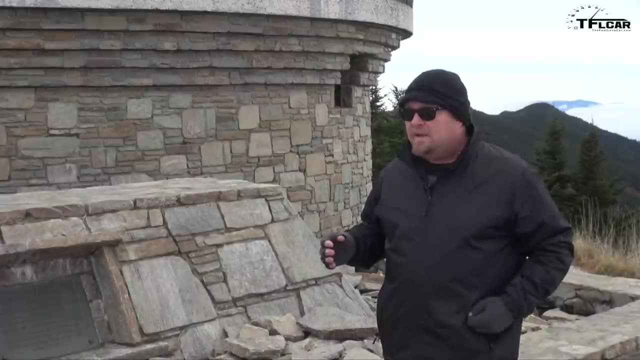 And I got to tell you, if you look around this place, I mean they've really done a number in terms of making it look absolutely pristine and modern while not really disturbing the nature around it. It's rather fascinating, And that goes for the entire area we've been. 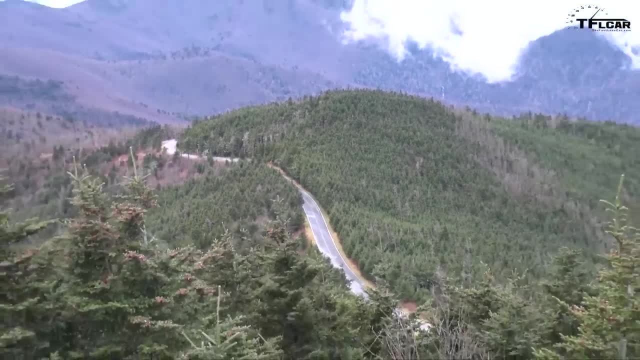 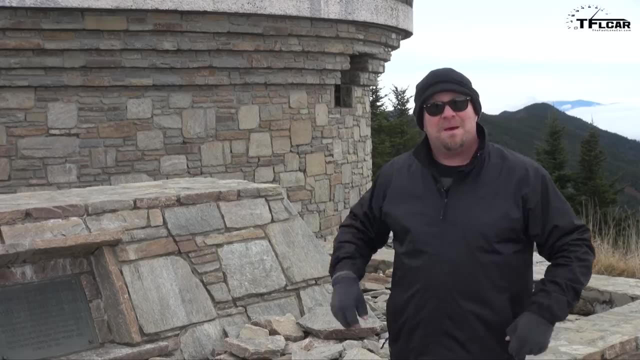 involved with here. The roads have been fantastic, Everything's been groomed perfectly. It's an amazing park with lots of amenities. but if you come this time of year, be prepared: Bathrooms might be locked. The time of year is on the line. 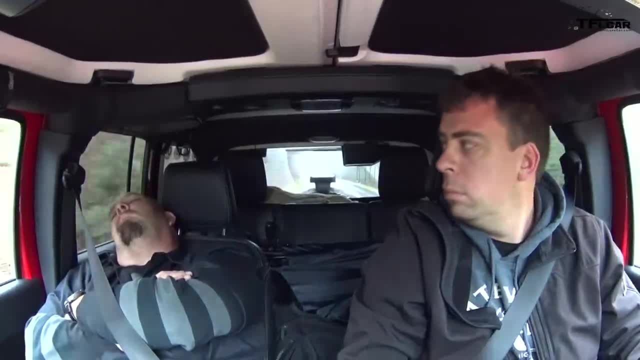 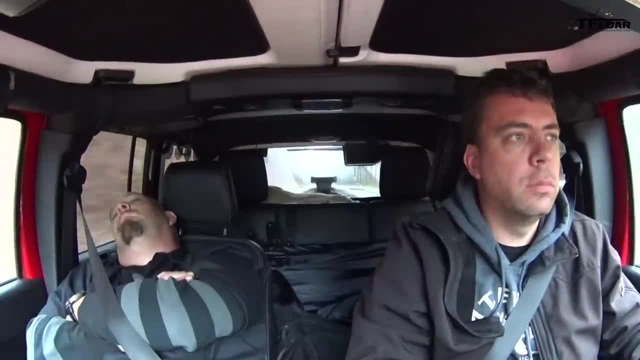 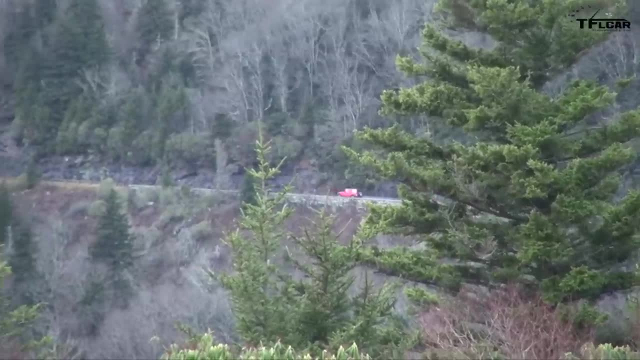 to driving around. The thing about this place is, when you go away for a bit, it's not that the laws of the world are all that much of a mess. There's just so many spaces that you can just walk around and you can just be going. 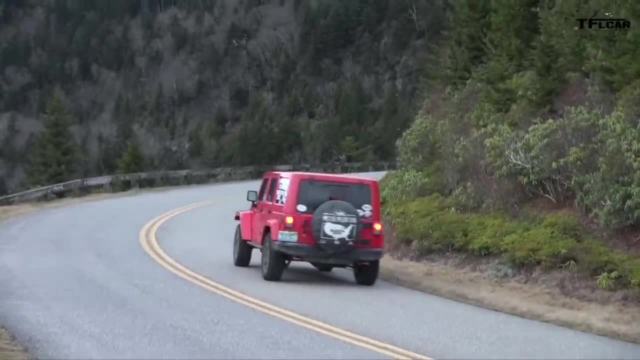 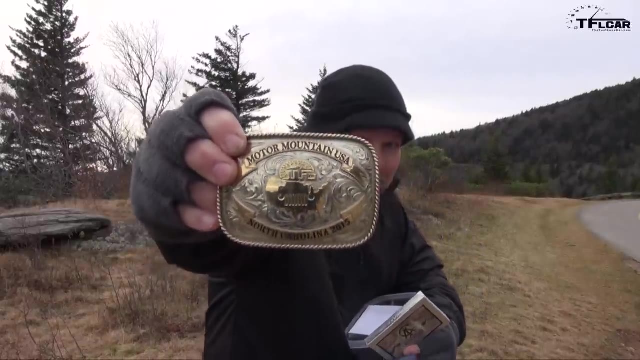 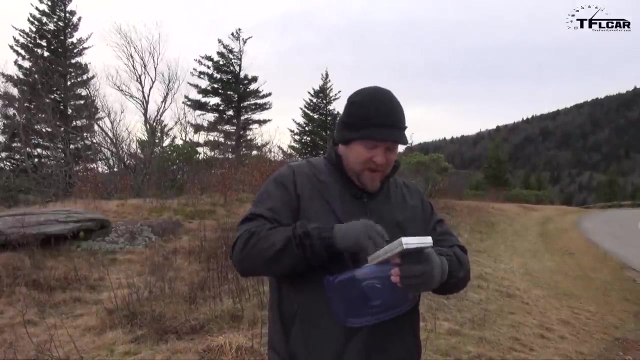 around in circles. It's been so beautiful here, That's right. All right, here we go, North Carolina. There's your buckle. Now, for those of you who don't know the drill, come to the coordinates. find this, which will be very easy to find: We're. 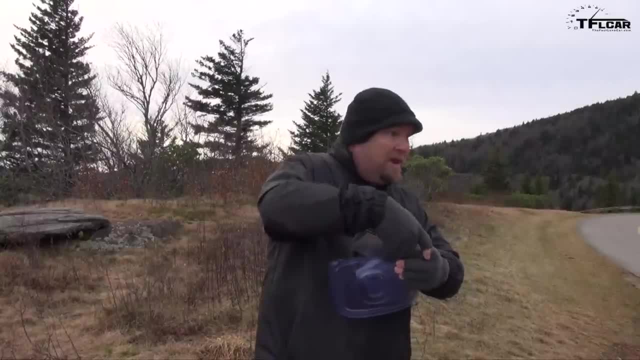 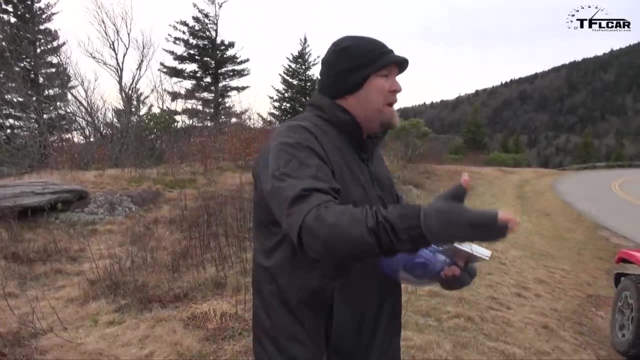 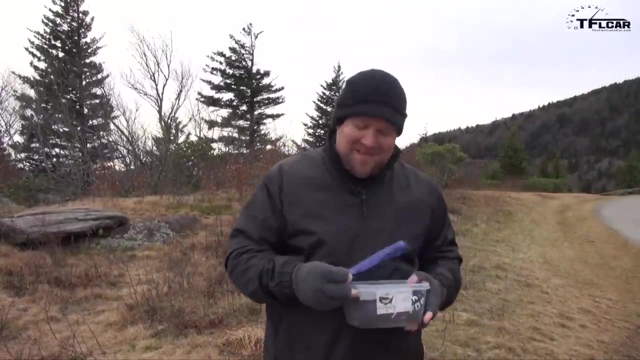 not too far away from Mount Mitchell and we're right off the Blue Ridge Highway. It's Parkway, It's a park. What is a parkway? What is a parkway versus a highway? Okay, okay. So when you find this, please contact the person on this card with a selfie of you and 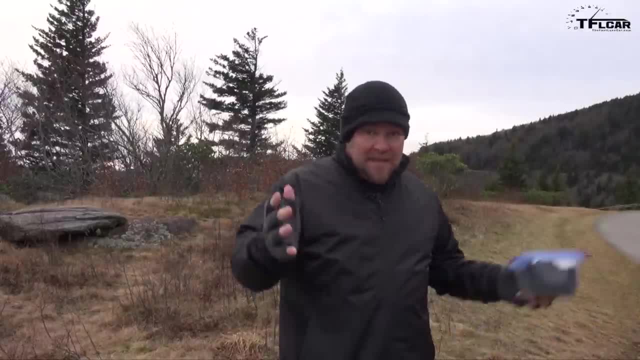 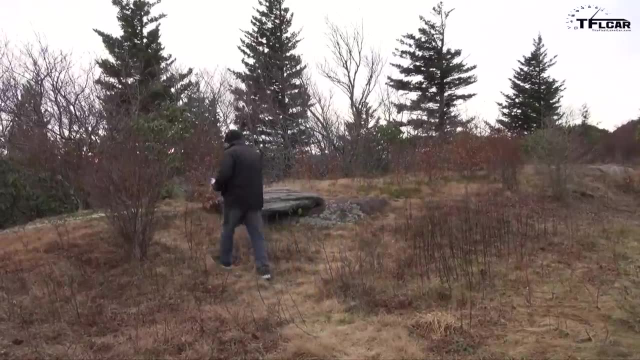 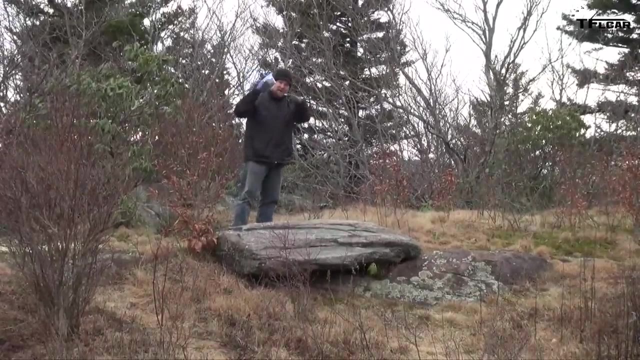 the boat buckle. If it's with a Jeep product, awesome. If it's not, that's okay. More importantly, we get your face with this Now. this is just off the road. There is this little kind of makeshift pathway here and giant rock, Giant rock. Yep, we're going to go in right here. 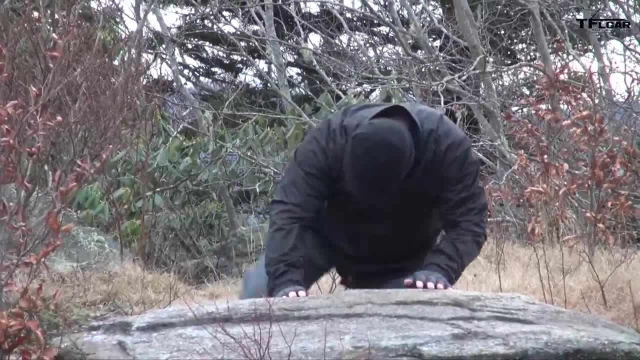 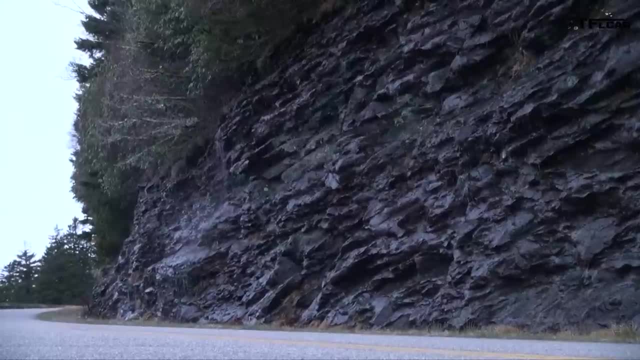 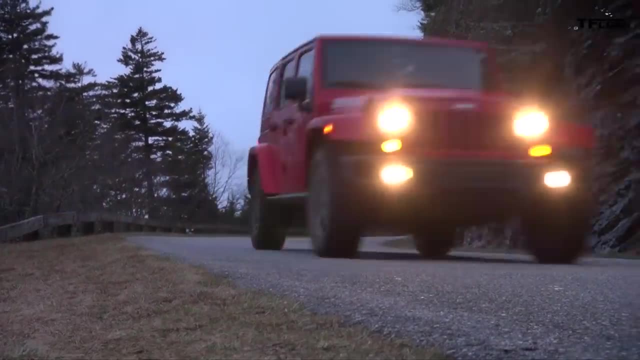 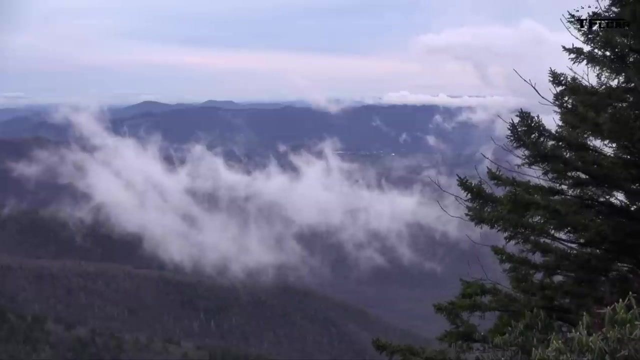 Just behind the giant rock. Let me see if I can get that in there. real good, Yeah, North Carolina, you have a beautiful state. This Blue Ridge Parkway is fantastic, Guys. we've been to so many mountaintops, but what makes this one so unique is seeing the way. 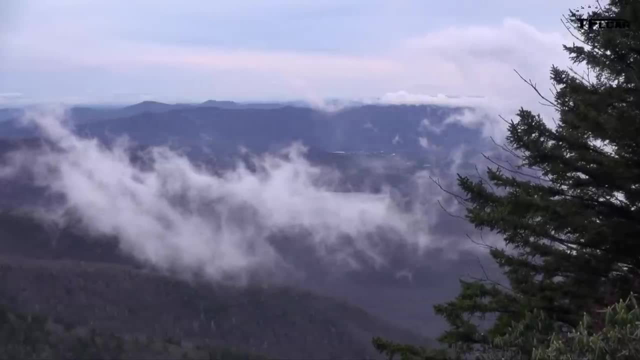 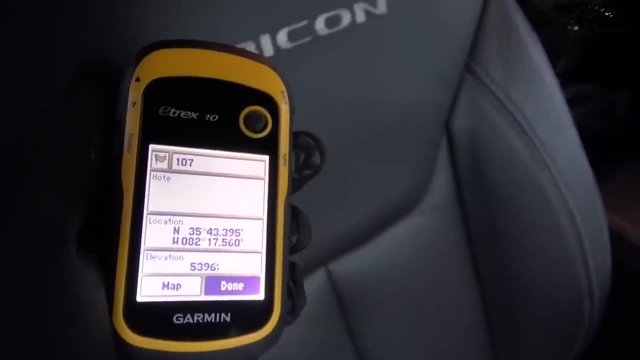 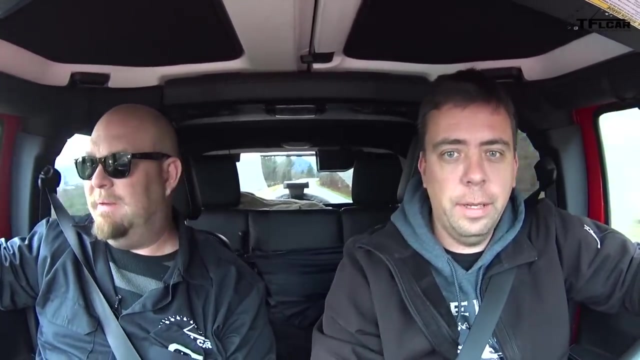 the clouds cling to the sides of the mountains, This amazing road And the green here. It's just astonishing. This is the highest mountain east of the Mississippi, 6,000 feet. Yeah, So we're actually higher right now than we are, at least, at our office in Boulder. 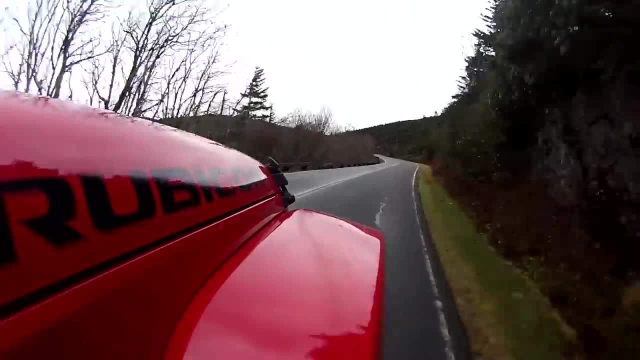 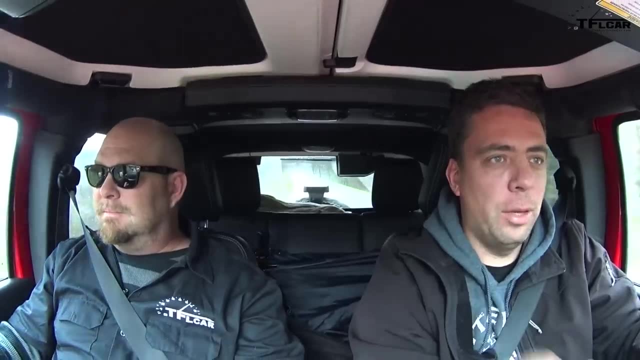 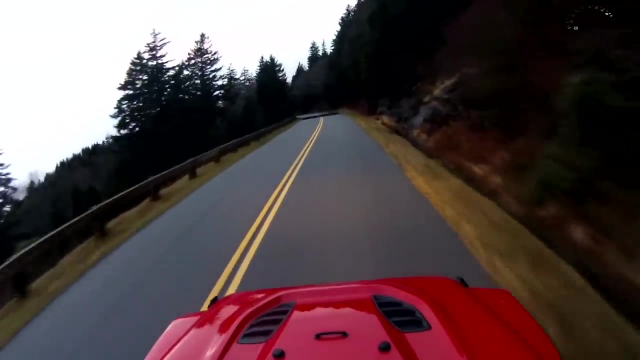 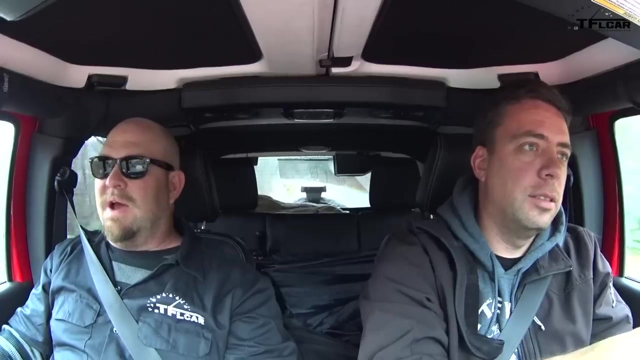 Right, By the way, the Tale of the Dragon is somewhere In this region as well. Yeah, Yeah, we're just going to fly down that in this, aren't we? We need a track hawk, Track hawk, Yeah, Track hawk Jeep. build the track hawk, Let us drive one on the Tale of the Dragon.